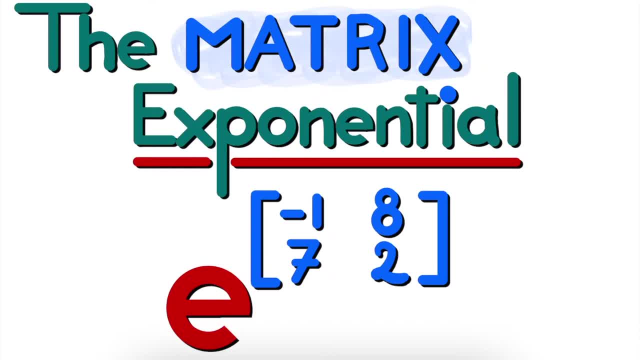 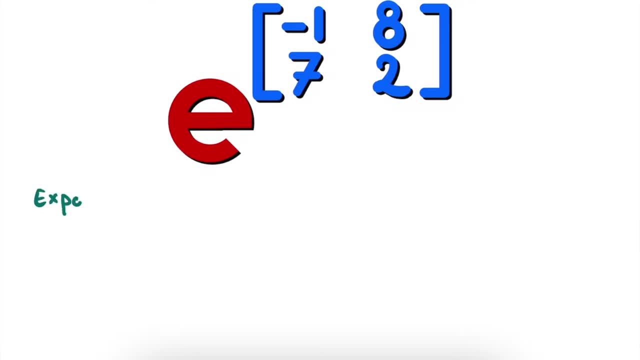 tool in quantum mechanics And therefore, if you want to understand quantum mechanics, you better know how to take the matrix exponential. We know, of course, what the exponential of a real number is. e to the power of x is simply a function which takes in a number. 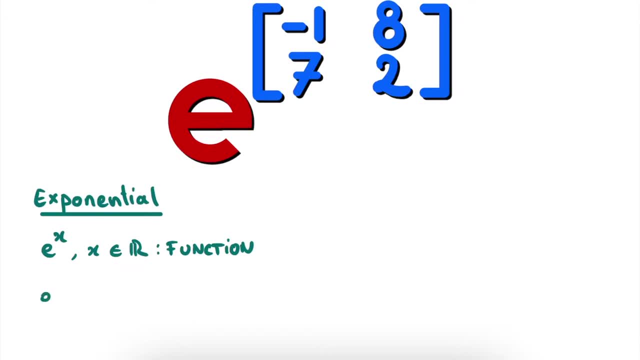 x and spits out another number. We even know how to take the exponential of a function of x, For example e, to the power of minus x squared, where minus x squared is simply another function in x And this entire e power is, in its own, again a function, Simply plug in. 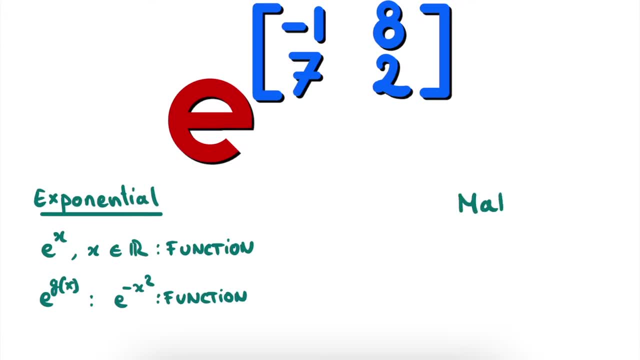 a number and you will receive a number back. And for matrices in particular, we know how to multiply them And therefore we also know how to calculate basic powers of a matrix. A, For example, A squared is simply A multiplied with A. A cubed is A multiplied with A. 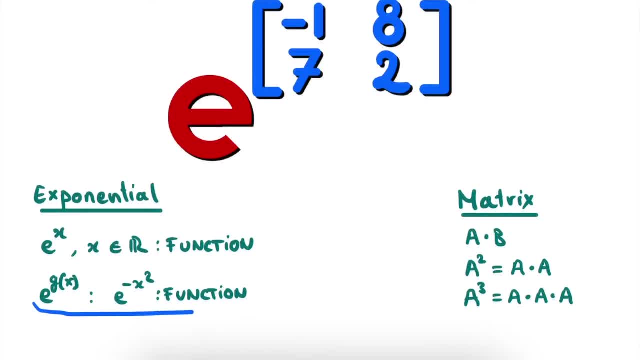 And so on. So, knowing these two fields in mathematics separately, how do we now combine them in order to calculate e to the power of a matrix? And that's what we'll turn to next, by solving an exercise step by step, where I explain everything I do along the way. 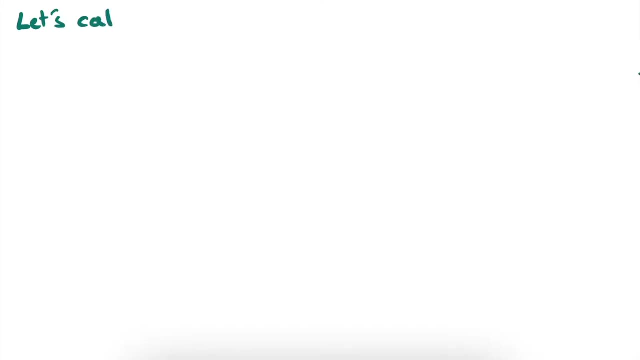 So let's do some calculations And, in order not to overcomplicate things, let's start with a 2 by 2 matrix. A is equal to minus 1.. 8,, 7, and 2.. And what we want to calculate now is e to the power of this matrix. So we 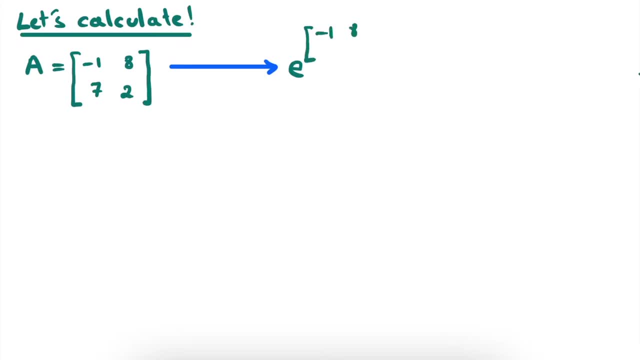 simply put this matrix in the exponent Minus 1,, 8,, 7, and 2.. And alternatively, you might see this written in the following way: Simply exp or exponent. open a curly bracket, then write your matrix So minus 1,, 8,, 7, and 2.. Close the matrix and close the curly bracket. 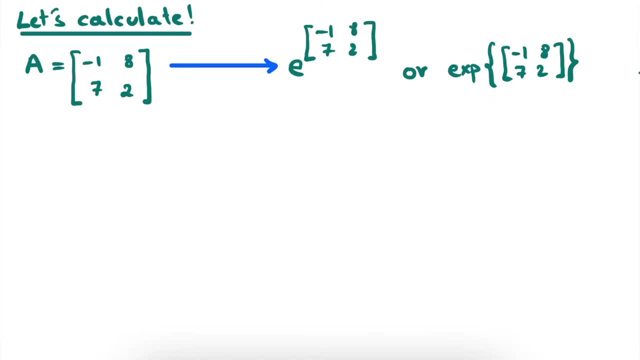 And this latter notation is, of course, to avoid writing this entire matrix as a superscript in the exponent. So let's now see how we actually calculate this thing, And the only piece of information you need in order to calculate this is that you have to take the Taylor series of the 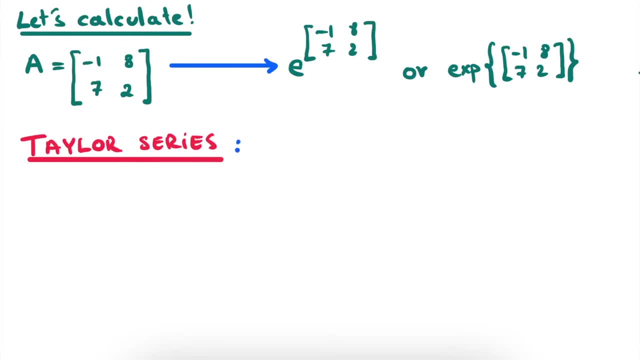 e power, And the idea behind the Taylor series is to write the function, in this case e, to the power of x as a sum of powers of x. So we have 1. Plus x Plus 1 over 2 factorial x, squared Plus 1 over 3 factorial x to the power of 3.. 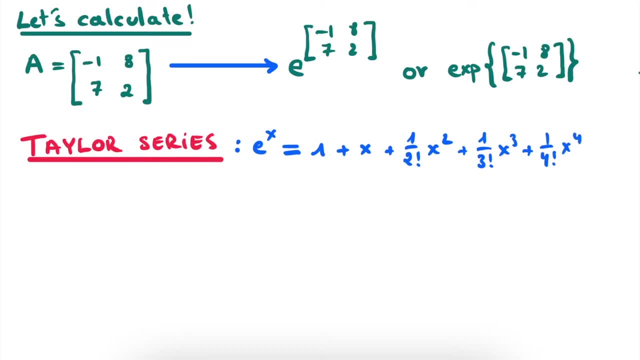 Plus 1 over 4 factorial x to the power of 4.. And of course by now you get the general scheme And we can write this in a more compact form using the sigma notation. We sum over the index k with x to the power of k in the enumerator and k factorial in the numerator. 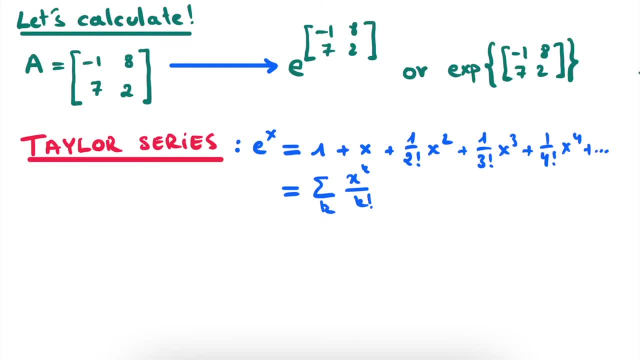 Alright, so now we have written e to the power of x as a sum of powers of x, And the crucial point here is that x is not constrained to being a real number. It can also be- you guessed it- a matrix. So let's see what this becomes. if we have e to the power of a, where a is a 2 by 2, 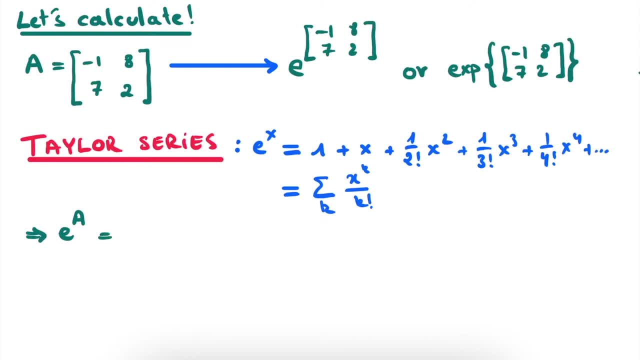 matrix, or any matrix really. Then we can write this as the following: We have 1,, which becomes the unity matrix, Which in our case will be the matrix 1,, 0,, 0,, 1.. The unity 2 by 2 matrix. 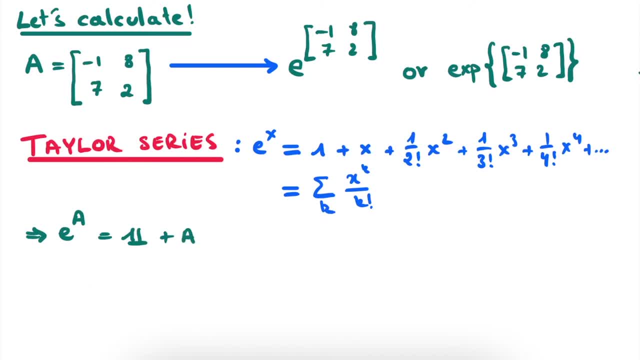 We add to this simply a, which corresponds to this x right here. But now a again is a matrix. Then we add 1 over 2 factorial a squared, And we know of course how to take the square of a matrix. It's just a basic matrix multiplication. We add to this 1 over 3 factorial a cubed. 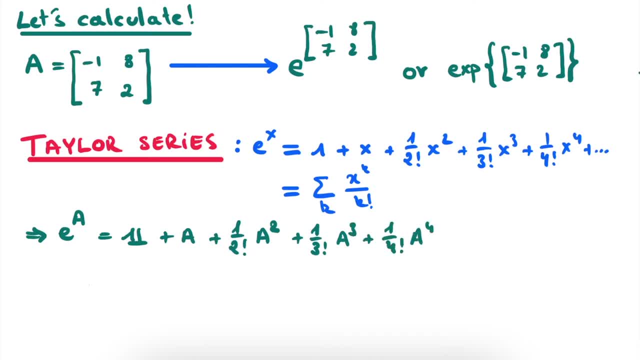 Plus 1 over 4, factorial a to the power of 4.. And so on and so on. And now you can see that in this simple way we've written the matrix exponential e to the power of a simply as a sum of matrix multiplications. So a to the power of 2, a to the power of 3, a to the power of 4,. 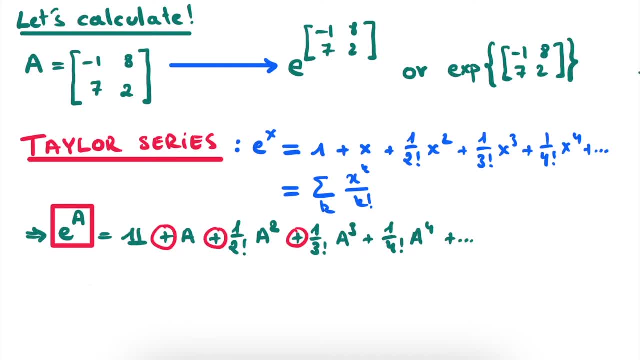 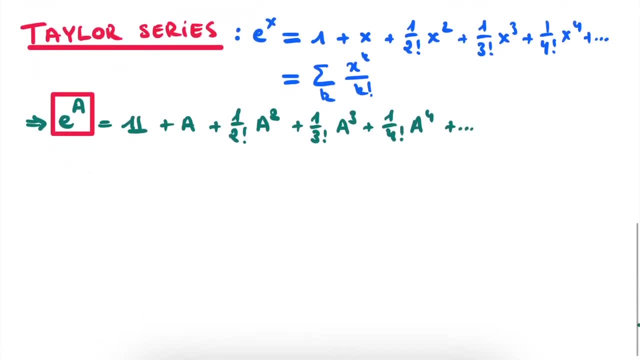 and so on, and so on. So the only thing that we need is to be able to multiply matrices and add matrices. So let's see how this now works out. for our specific exercise, We had e to the power of the following matrix Minus 1,, 8,, 7, and 2.. And now we will rewrite this: 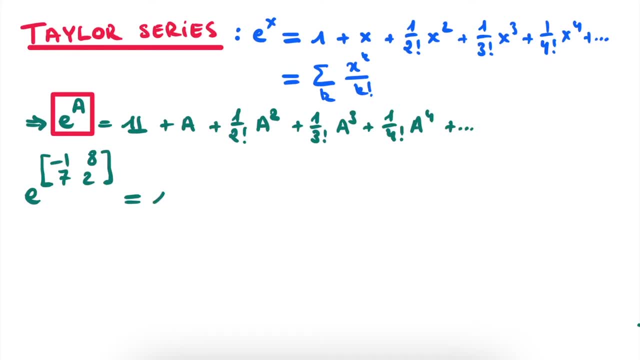 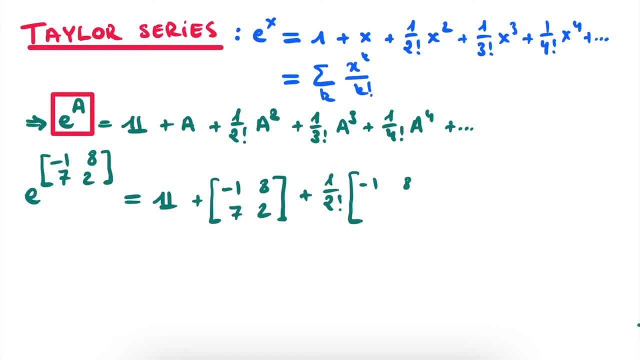 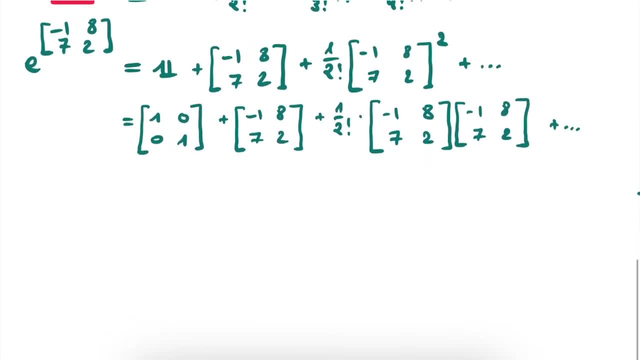 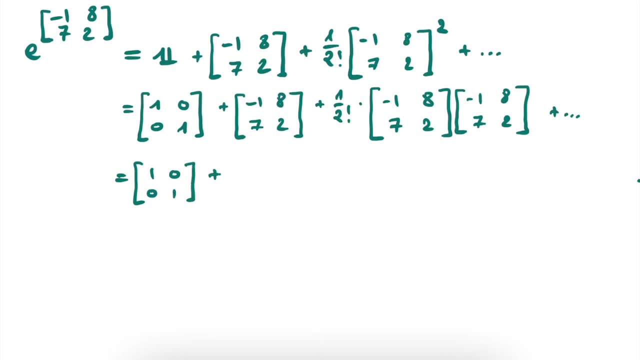 other terms, and let's now simply do this matrix multiplication. so we have again copying the unity matrix plus our matrix to the power of one, but that's simply our matrix, again plus one over two, multiplied with the multiplication of these two matrices- and if you're not sure about how to multiply matrices, I 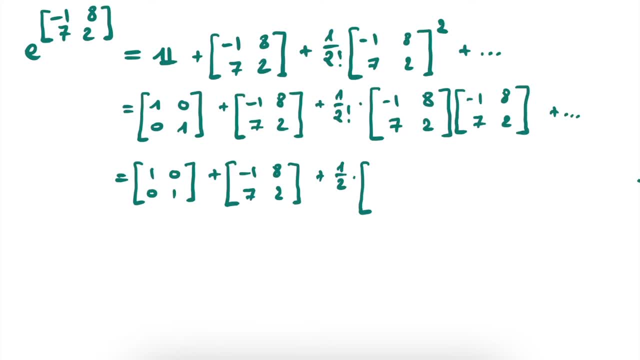 gladly refer you to a video where we solve exercises specifically on multiplying matrices step by step. so let's see what we have here. so for our first element, we have these two numbers multiplied and we add to that these two numbers multiplied and this gives us 57.7. 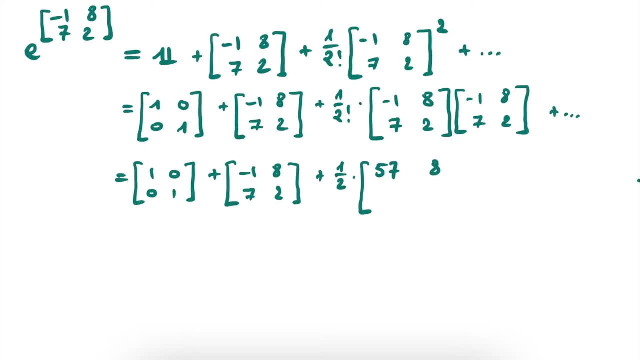 for the second element, we get eight, for the third element, we get seven, and for the fourth element, we get 60, and we of course add to this all of the remaining terms where we have to cube the same matrix, and so on, and so on. and now comes 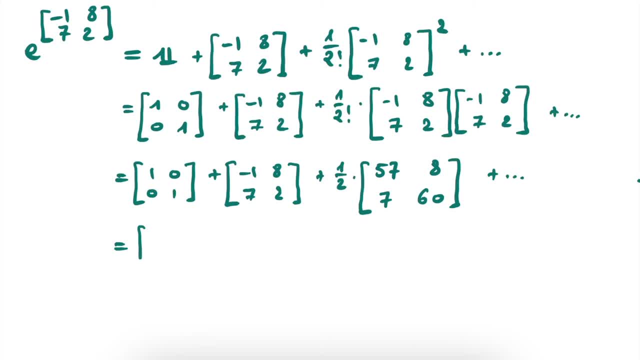 a step where we add all of these matrices together. so for the first element, we have one minus one plus 57 divided by two, which of course gives us a step where we add all of these matrices together. so for the first element, we have zero plus eight plus four, because we have to multiply this eight by this one. 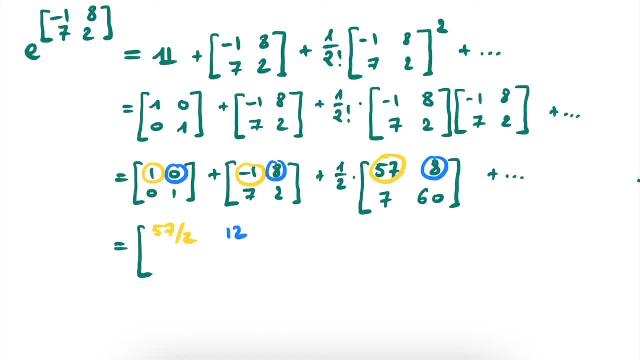 half in front, and this of course gives us twelve. then we have zero plus seven plus three and a half, which gives us ten point five, and then the last element, we have one plus two plus sixty divided by two, which is thirty. so we get the last element, thirty two, and this matrix needs of course to be added. 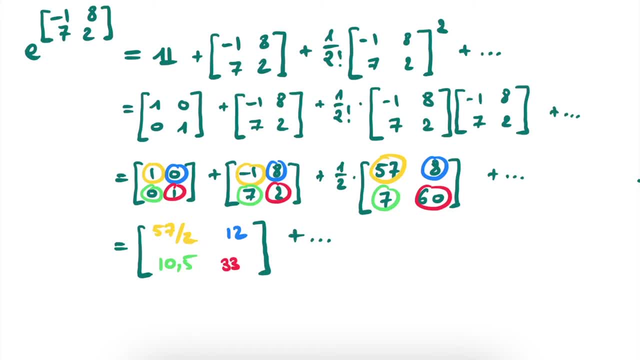 with all of the other matrices that you have. and well, this is exactly an infinite number of matrices that you need to add, but since most of the time, this is infeasible to do, you can simply put this wiggly sign above the equality sign to. 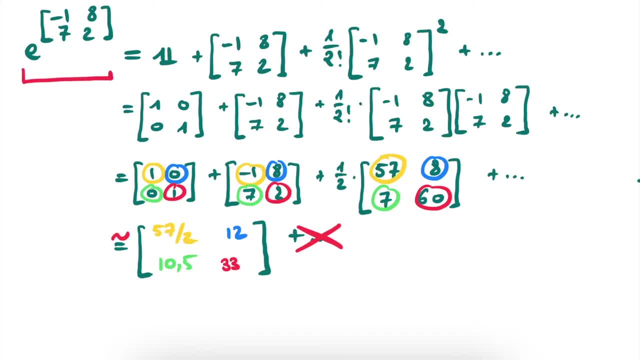 show that e to the power of this matrix is approximately equal to this matrix right here, and it's of course important to address that. we only get an approximate result here, which could be experienced as quite unsatisfactory. however, by using this general approach, this will oftentimes be the outcome and you cannot do anything. 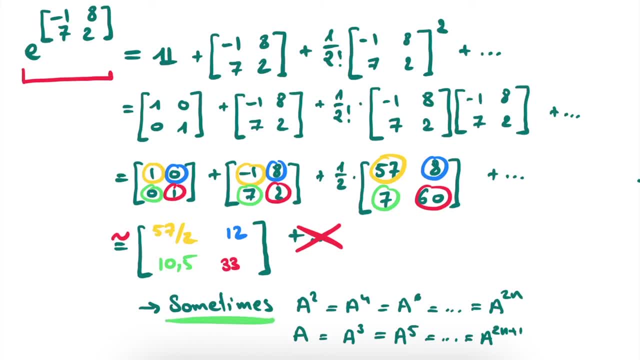 further, however, sometimes for very specific matrices: a, you have the fact that a squared is equal to a to the power of four, a to the power of six and, in general, that all of the even powers of a are equal to each other, and likewise you will have that all of the odd powers of 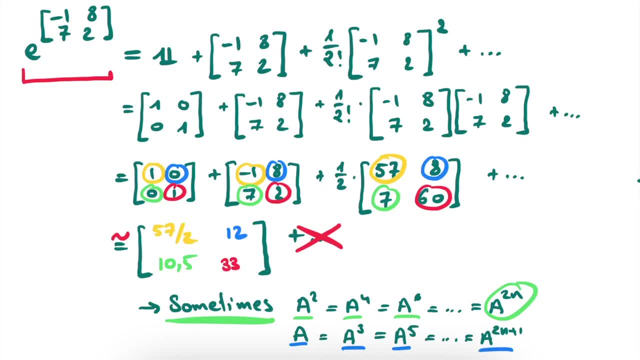 a are also equal to each other, and this will make it so that all of these other terms can be collapsed towards just a handful of matrices, and in that case you might be able to get a closed form solution without needing to get this approximation. however, for the 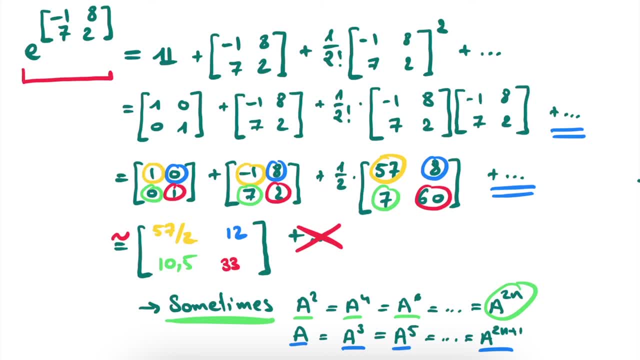 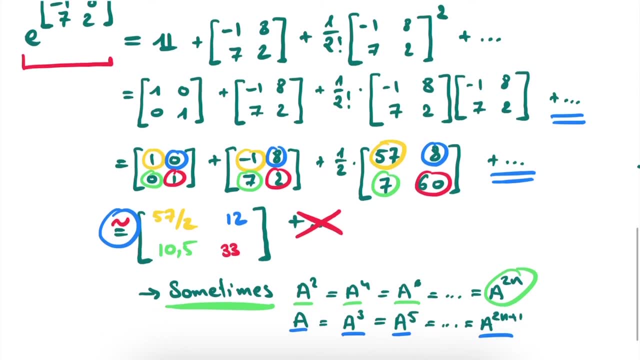 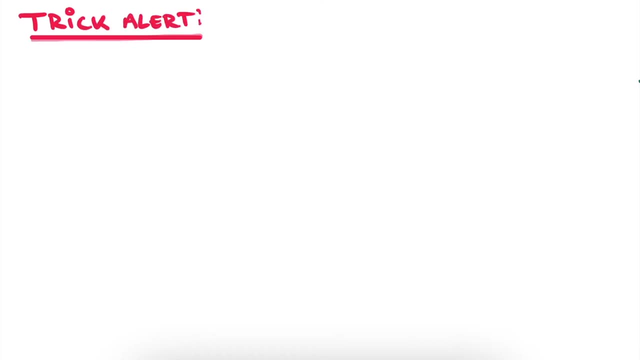 majority of matrices, this property will not be true and therefore it's good to know that most of the time, you will indeed get an approximate result. however, if you really do not want to settle for an approximate answer, then there is one more trick that you can do, and 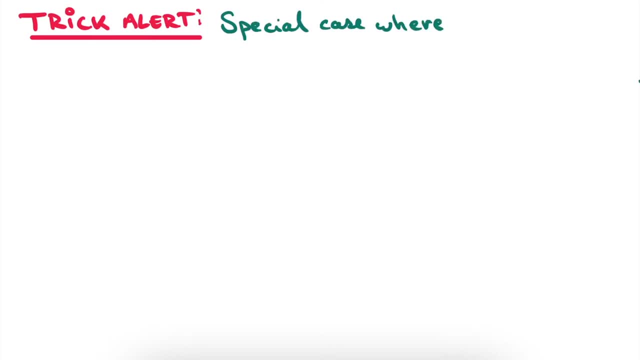 this trick builds around the fact that this matrix exponential becomes very simplified. for diagonal matrices we have the property that if a is diagonal- and let's take, for instance, a diagonal two by two matrix with elements alpha, zero, zero, beta- that we have that e to the power. 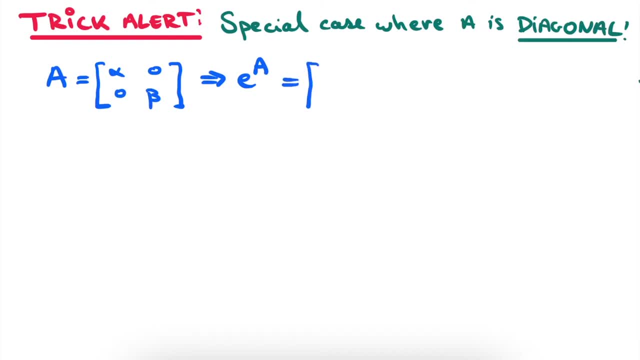 of a. so the matrix exponential simplifies to the following: e to the power of alpha for the first element, zero, zero. and e to the power of beta for the fourth element. and we see in this case that the exponential of this matrix is simply transferred to the diagonal elements of this. 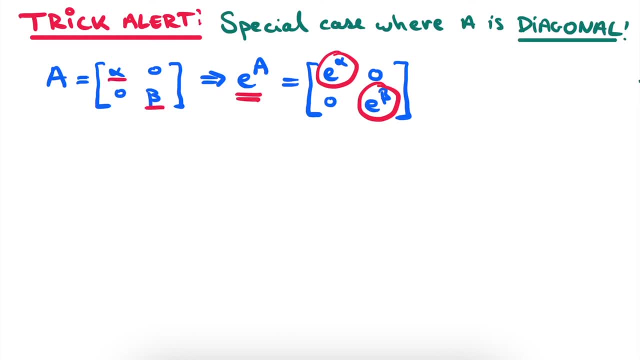 matrix, lifting each of the diagonal elements to the exponent. now, just to stress here and to make sure that you don't make any mistakes, is that this is only valid for diagonal matrices. if you do this for non-diagonal matrices, then you will make a mistake and the result will not be correct. now. 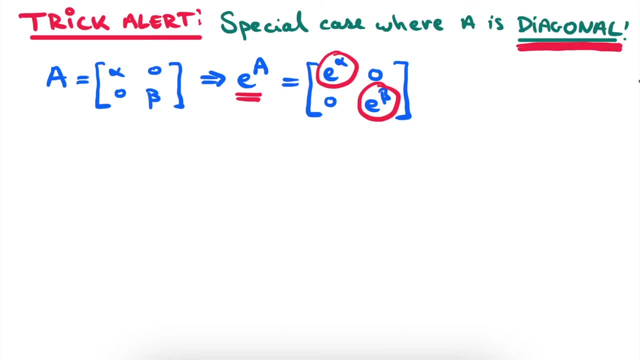 you might, of course, object that not all matrices are diagonal. however, there is a procedure that you can do to make matrices diagonal, and this is called matrix diagonalization, and it is actually a central mathematical process that is done in quantum mechanical calculations. And to end off, let's prove this property for diagonal matrices as an added practice. 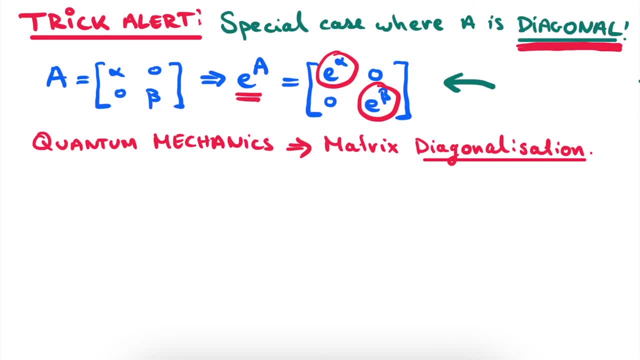 exercise of this Taylor expansion method. So we have that e to the power of a is equal to the unity matrix plus a plus one over two. factorial a squared plus one over three. factorial a to the power of three plus all of the other terms Writing down the matrices we find for this. 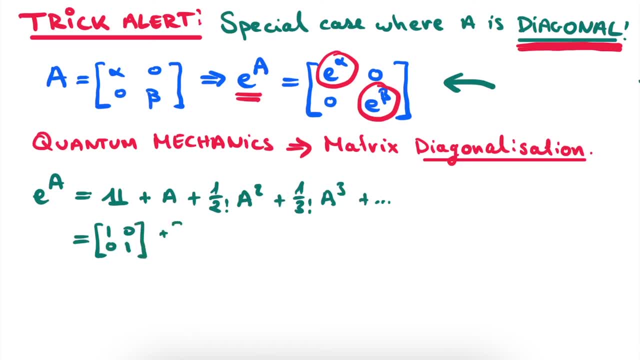 first one, 1, 0, 0, 1, plus the diagonal matrix alpha 0, 0, beta, and alpha and beta can be any number you like, plus one over two factorial times this matrix squared, so alpha 0, 0, beta squared plus one over three factorial. 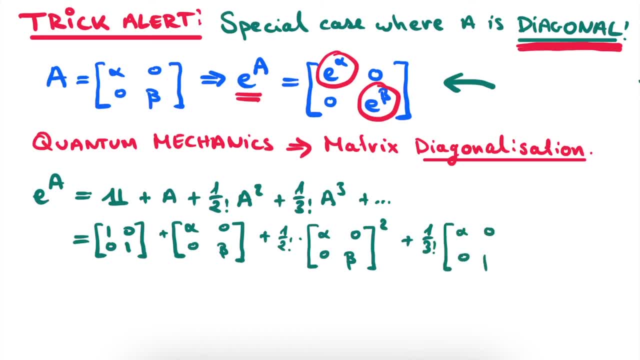 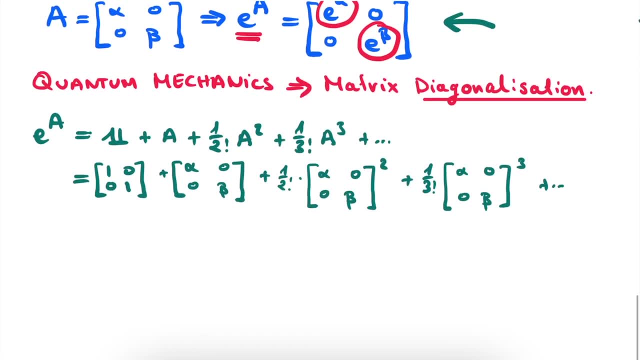 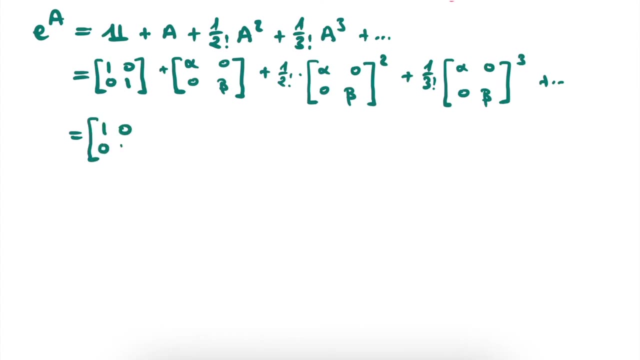 now supply by alpha 0, 0 beta to the power of 23 and so on for all of the other through terms. So let's now do this matrix multiplications and see what the exact get. so we have, of course, still these first matrix: 1, 0, 0, 1. plus we still have our original matrix, alpha 0, 0. 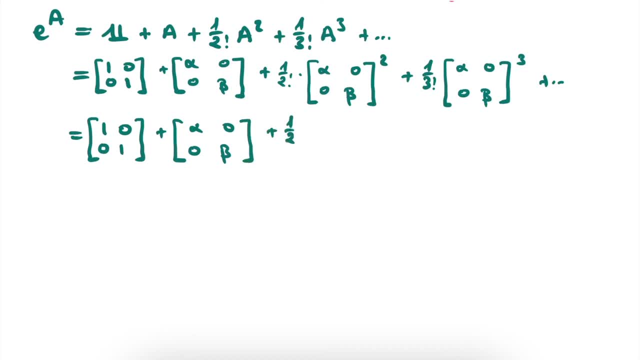 beta Plus one over two, and then we multiply these two matrices together by doing a matrix multiplication, of course. so we have alpha 0, 0 beta for the second matrix and then for the third one we have 1 divided by 3, factorial of alpha 0, 0 beta. 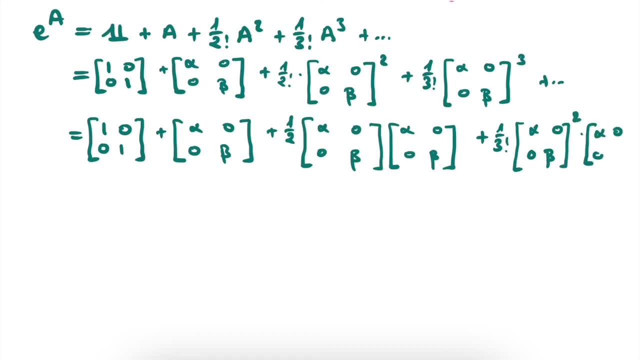 squared multiplied by alpha 0, 0 beta. and of course we do not forget all of these other terms. and so let's now do this matrix multiplication after we have copied these matrices right here. so alpha 0, 0 beta plus one half divided by well, multiplying these matrices, we have alpha squared. 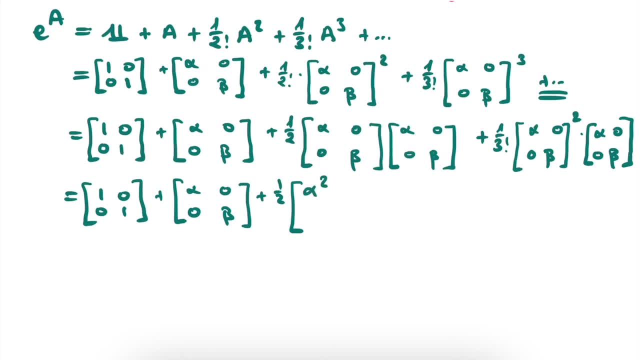 plus zero. so for the first element, we simply have alpha squared. for the second element, we have alpha times zero plus zero times beta. well, this is of course zero. same for the third element. and for the second element. we have alpha times zero plus zero times beta. well, this is of course zero. same for the third element and for the 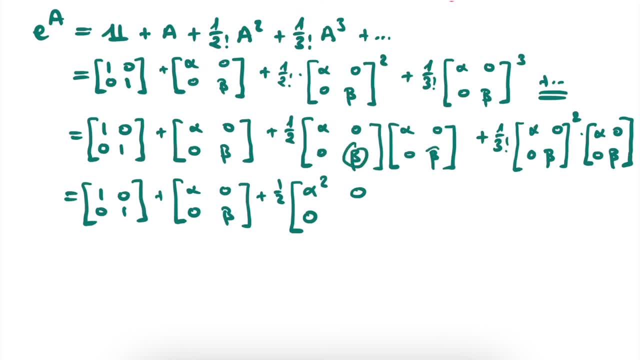 fourth element: we have zero times zero plus beta times beta, which is, of course, beta squared, and we see that this matrix squared is simply the square of its elements, and which is a property that only holds for diagonal matrices. using this, we can now write down this third power, because we know that. 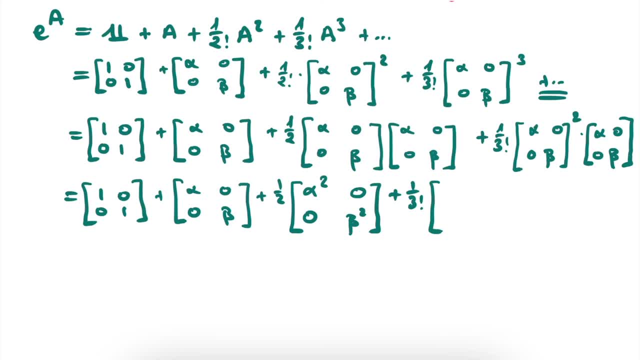 the square of our original matrix is simply the square of its elements. we have alpha squared, zero, zero, beta squared and we multiply this with our matrix- alpha, zero, zero, beta- and we add all of the other terms. now, if we do this multiplication, we again get alpha squared times alpha plus zero. 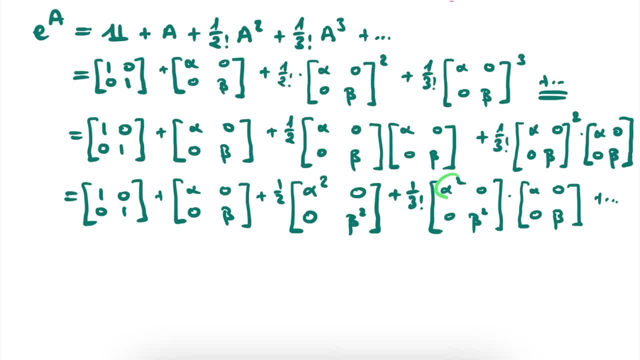 which is of course alpha cubed. for the second element, we have alpha squared times zero plus zero times beta, which is zero. the same is true for the third element. for the fourth element, we have zero multiplied by zero plus zero, just beta squared multiplied by beta, which is of course beta cubed. so we can already remove this. 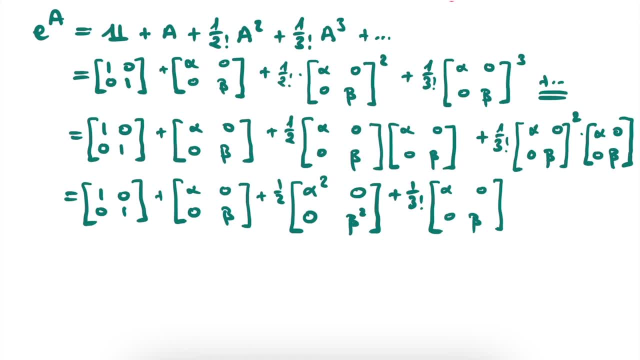 one right here and these powers here get lifted by one. so we have three and three and all of the other terms of course, and this pattern that each time the power of this matrix drops down to the elements of this matrix, will be true for any power. so if we then do the step where we add: 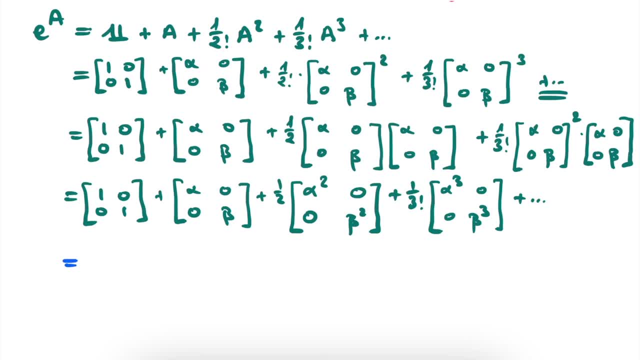 all of these matrices together, we get the following very large matrix: we get one plus alpha, plus one over two alpha squared, which is of course this term, plus one over three factorial alpha to the power of three, which is this term plus all of the remaining terms which. 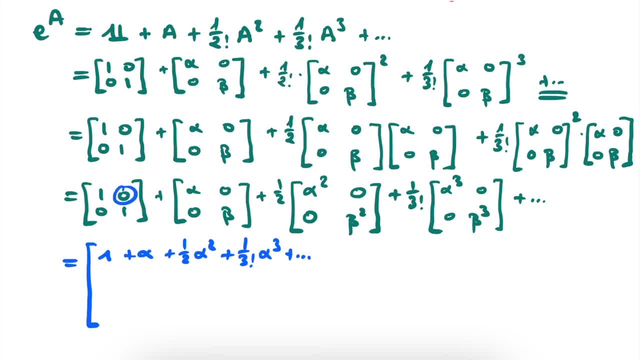 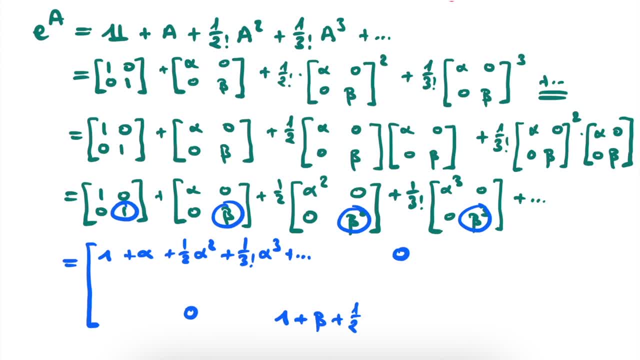 plus beta plus one over two, beta squared plus one over three, factorial beta, cubed plus, and so on and so on, and what we see now is that for these diagonal elements, we actually have the identical series that we had right here, but now simply with the elements alpha and beta.